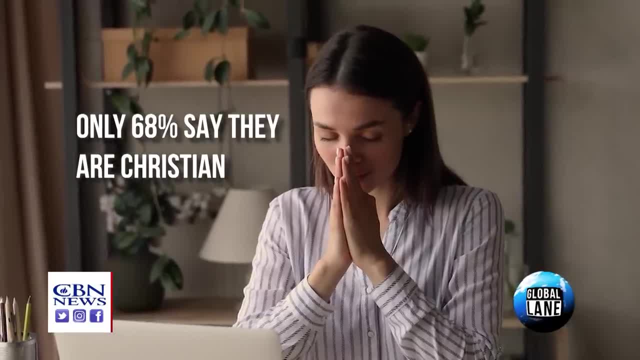 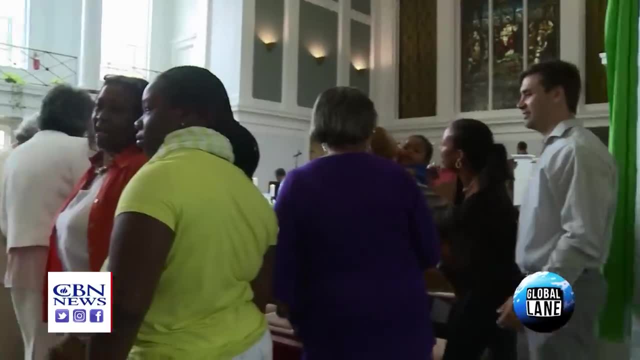 its skid. over the last number of years. We've gone down below the 70 percent mark. now We're down at 68 percent. So for a nation that used to have more than nine out of 10 of its adults who at least claim to be Christian, now down to two out of three. 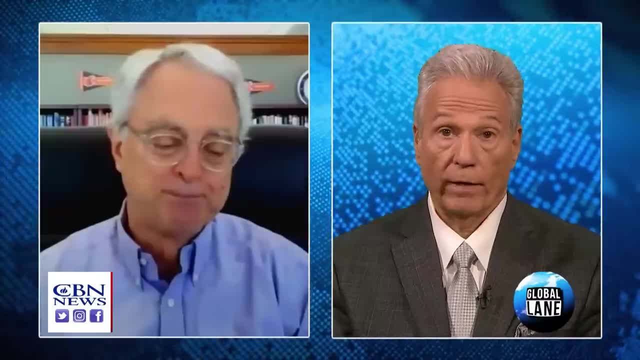 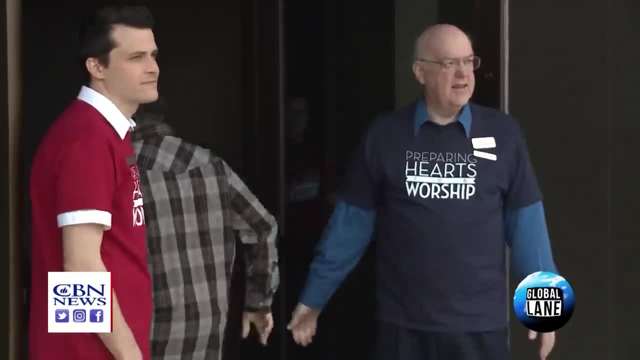 that's something that we need to pay attention to. And what I found most shocking, George, was your finding that only 55 percent of evangelicals believe that people are born sinners and can only find salvation in Jesus Christ. Did that shock you? This is a 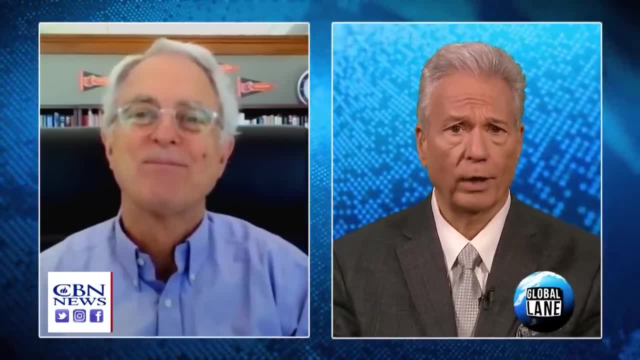 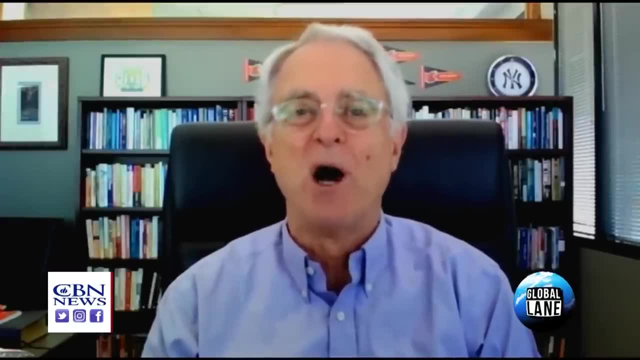 core evangelical Christian belief. Why do you think the church is faltering on that? Well, there are some things that we know that even evangelical churches tend not to talk about very much. Sin is one of those issues. The reality of Satan is another one of those. 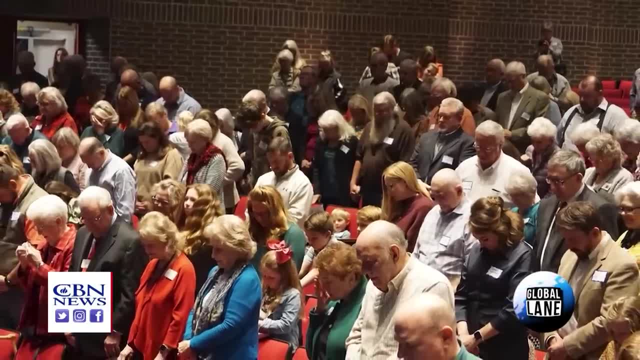 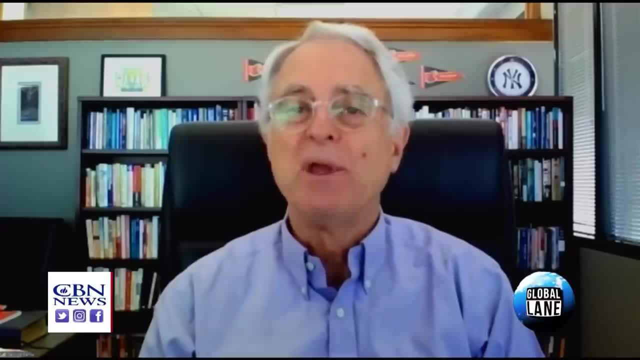 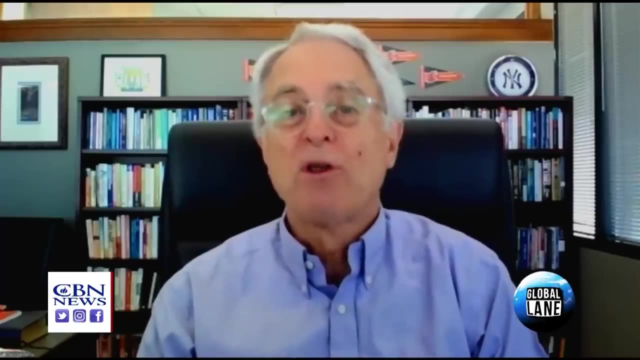 issues. When you start putting together the variety of things that evangelical churches, much less other Christian churches, don't talk about very much, you can begin to see why these patterns emerge. And so you've got that. And then also look at the fact that a third of the people 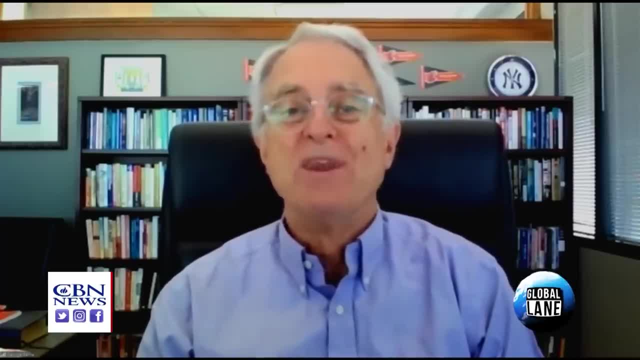 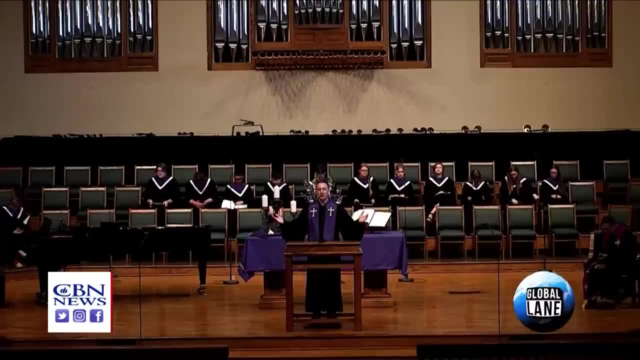 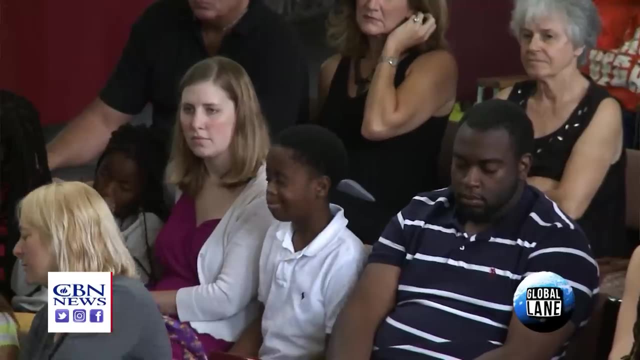 who sit in evangelical churches every week would not probably qualify as born-again Christians. Only God really knows, But the research simply tries to estimate where do people stand spiritually And when we ask people what they think will happen to them after they die, and we find that a third of the people that regularly attend evangelical churches 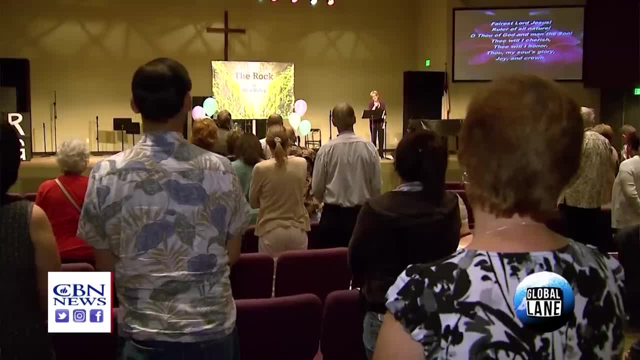 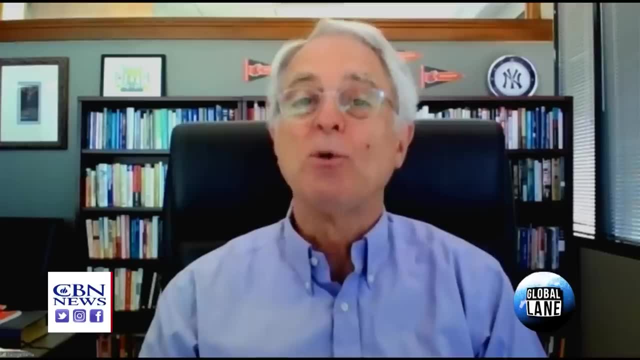 do not believe that after they die, they're going to go to heaven and only because they've confessed their sins and accepted Jesus Christ as their Savior. that too is a core evangelical perspective, But you've got a large share of the people in those churches that don't buy it. 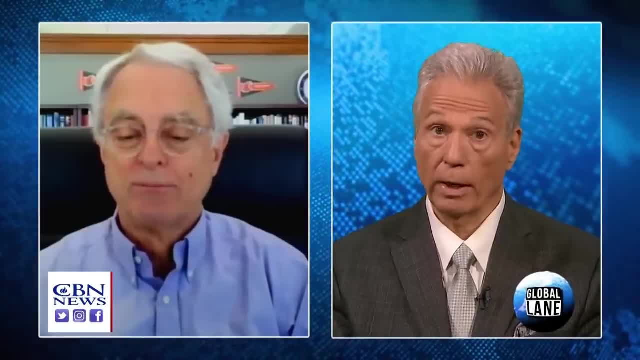 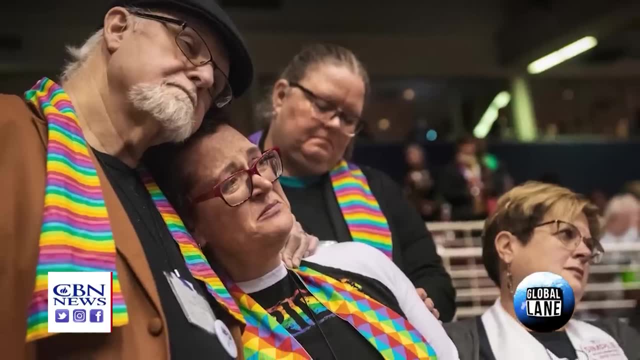 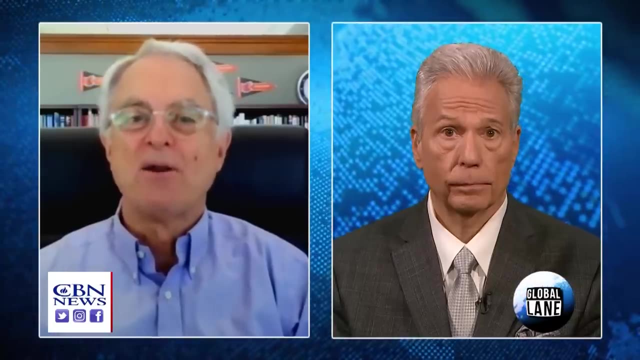 And you've been doing this for a long, long time. I know you've been doing this for many years, So does any of this surprise you? or do we see the culture starting to creep into the churches, rather than the churches influencing the culture? Yeah, honestly, this is a pattern that we started seeing about a quarter. 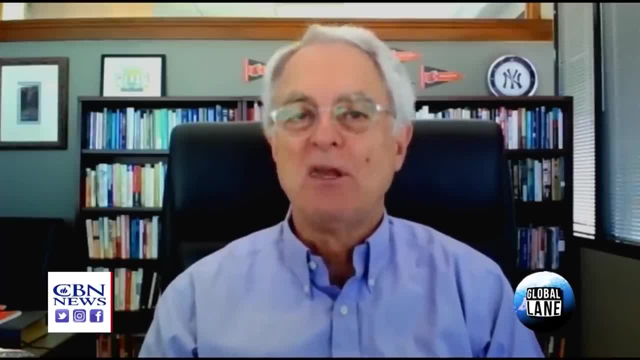 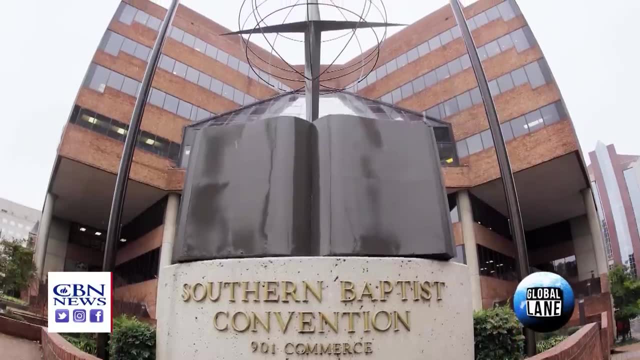 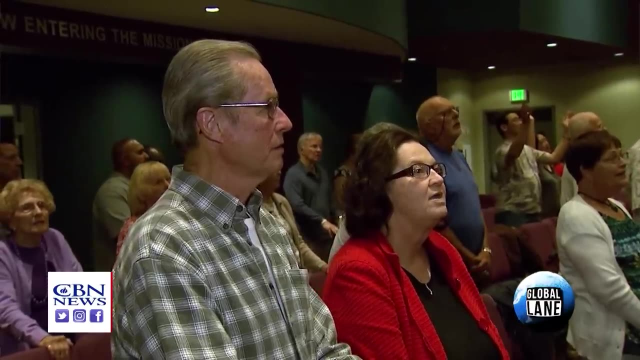 of a century ago, and it has simply continued. In evangelical churches it's been a much slower decline than, say, in mainline churches or other Christian churches, But nevertheless that decline has continued, And the pandemic was one of those opportunities. 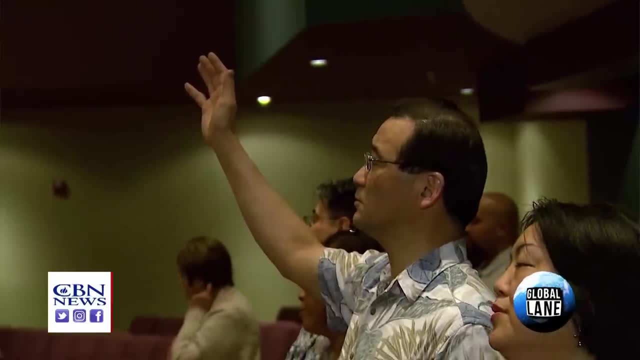 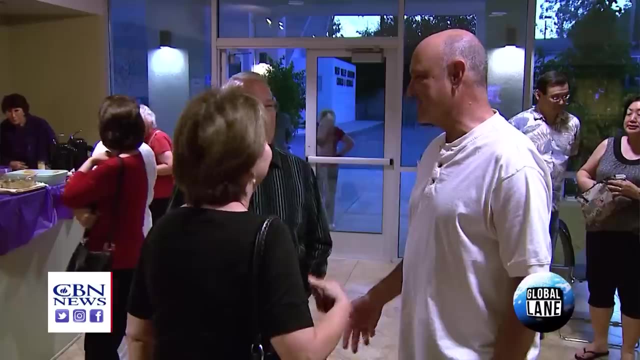 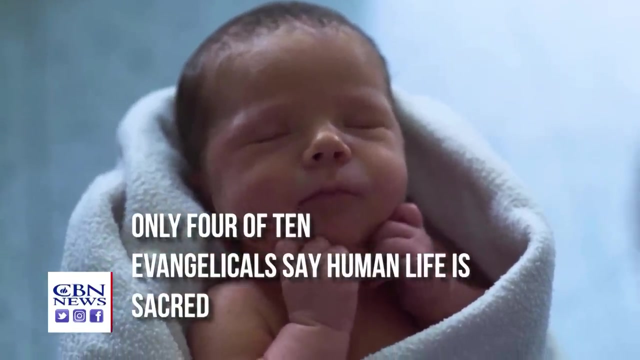 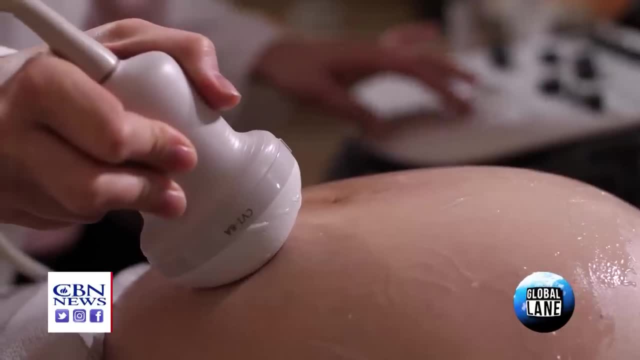 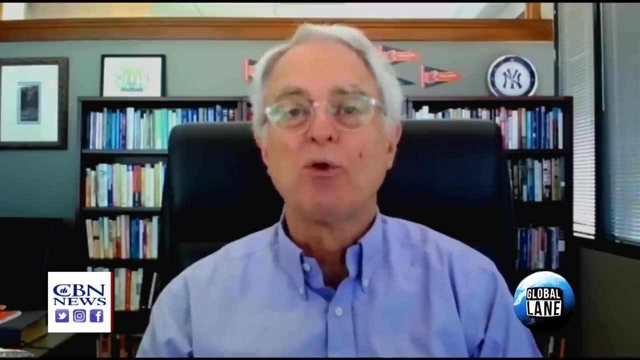 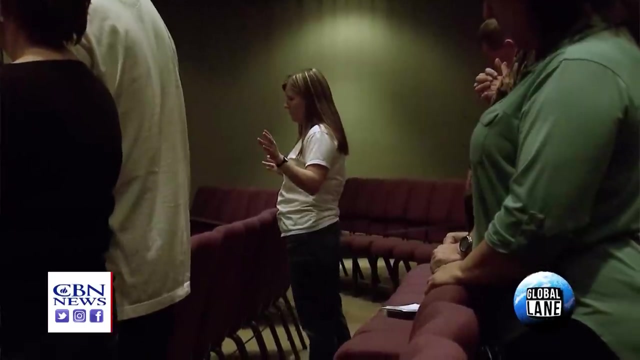 saying that abortion for any reason other than to spare the life of the mother or the child is morally unacceptable. So there's rampant biblical confusion or resistance, even in evangelical churches across the country. So what are the consequences of this then, not only for the church but our society as well, of this decline in core beliefs and 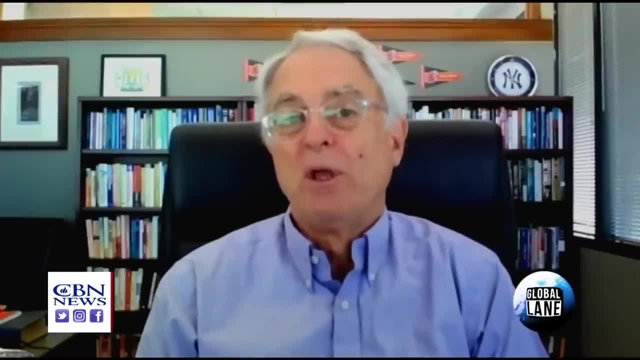 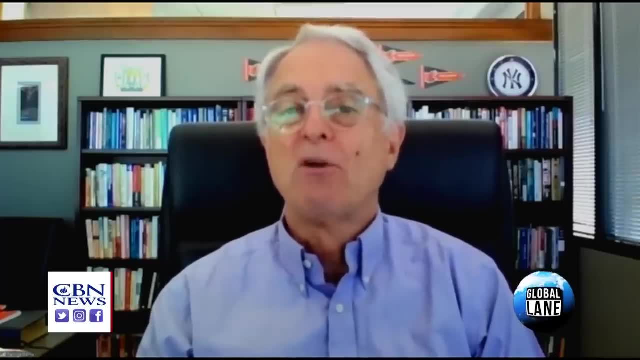 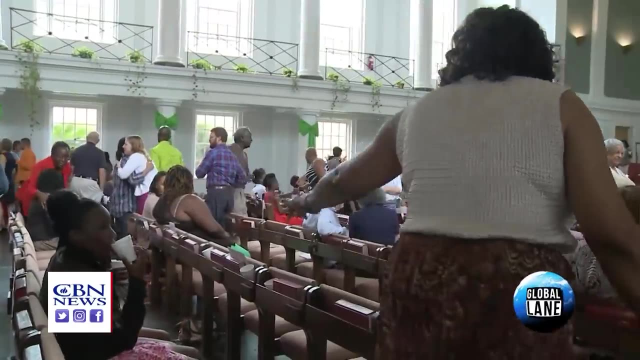 attendance continues. Well, one of the things that we could suggest is that evangelical churches- churches- are losing their theological distinctives. As far as the public is concerned, now, one Christian church is pretty much the same as any other, and it's hard to find evidence that that's. 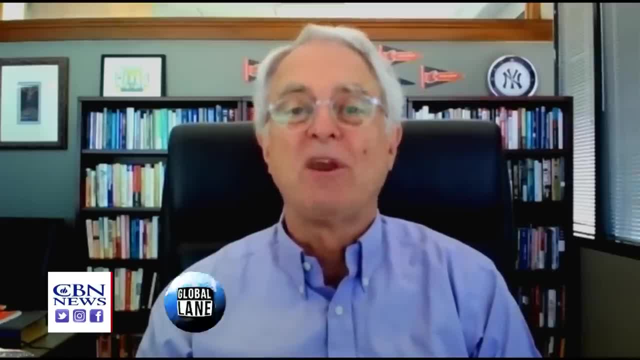 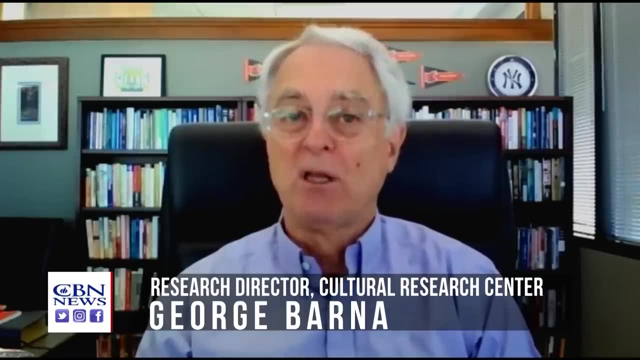 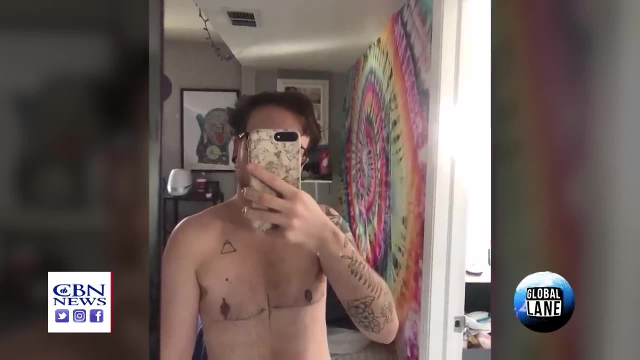 not the case Culturally. I think the scary part is that when you look to that group of people in our nation who can stand up biblically against many of the unusual, bizarre, immoral changes that are being proposed in public policy, that are being taught in our public schools, 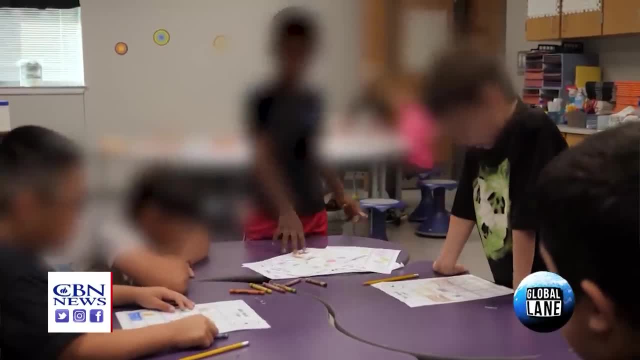 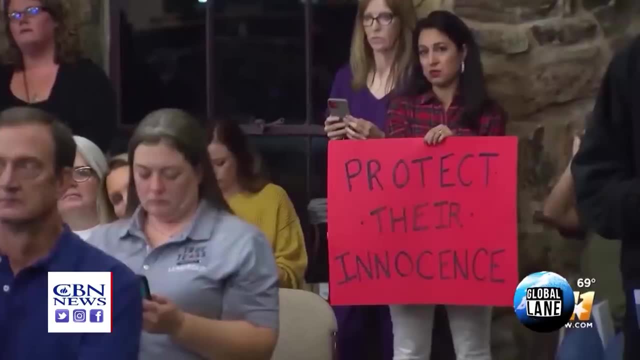 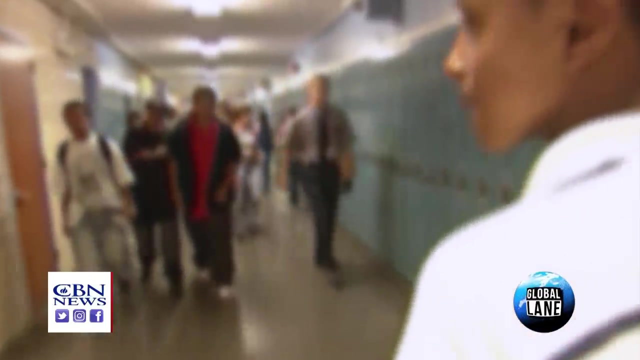 that parents are wrestling with as they're trying to figure out how to raise their children. In all of these areas, we're finding fewer and fewer people who embrace biblical perspectives, fewer and fewer people who are capable of defending biblical perspectives in the public square. 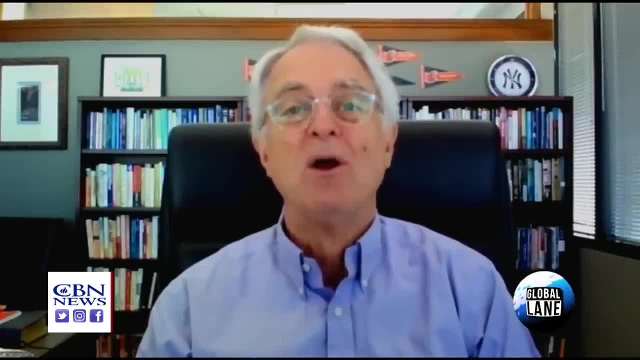 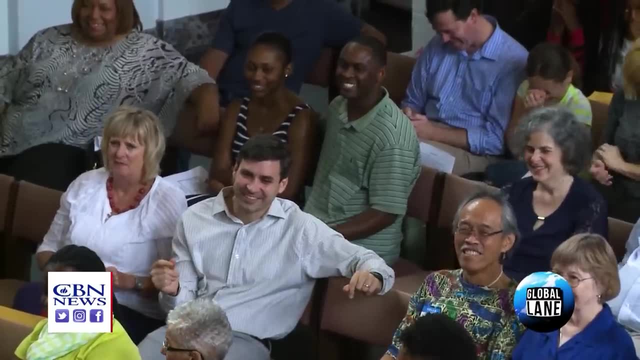 And so it's one of those situations, I think, where all of us need to sit back and say, wow, am I part of the problem or part of the solution? And if I'm part of the solution, how committed am I to being out there in the marketplace? 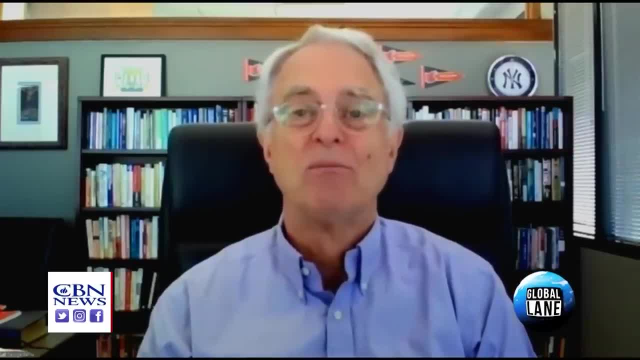 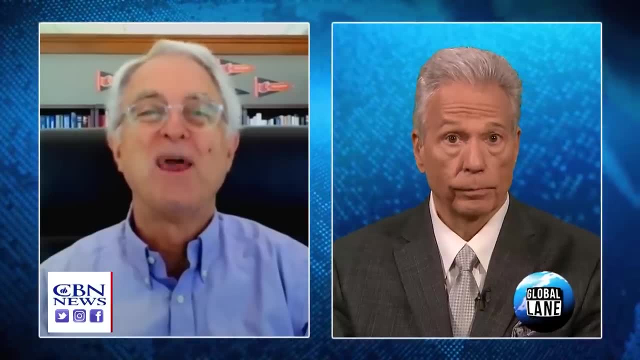 being that solution on a daily basis. Okay, salt and light. George Barna of ACU's Cultural Research Center, thank you for taking the time to share those insights. We appreciate it, George. Thank you so much.